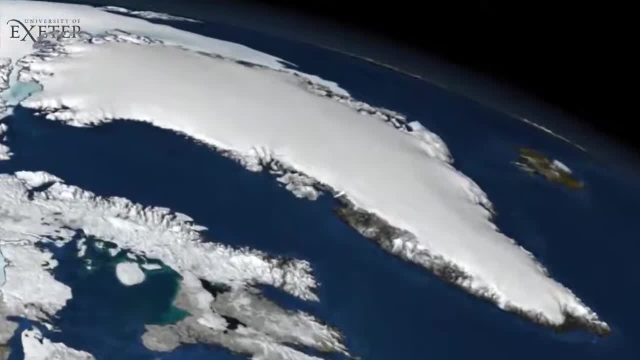 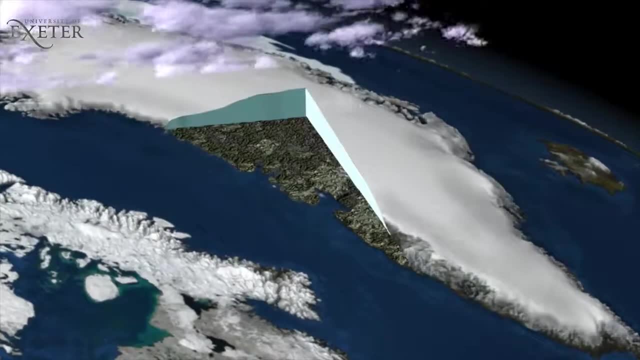 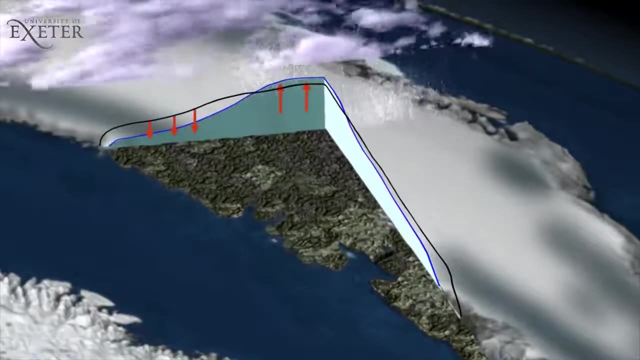 it was thought that, in a warming climate, both melting around the margins and precipitation in the interior would increase, causing the ice sheets to grow in the middle and shrink at the edges. It was thought that an increase in snowfall will offset the melt at the margins and there will be no change in how the ice flows, the ice dynamics. But 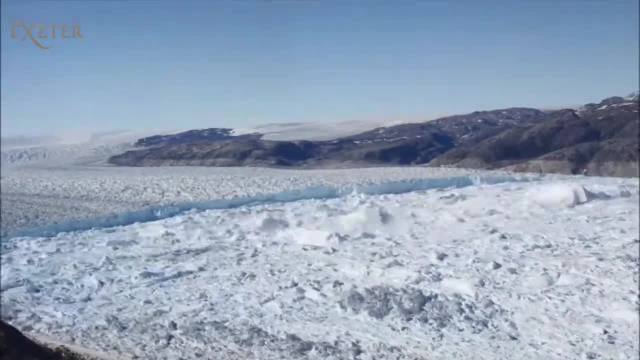 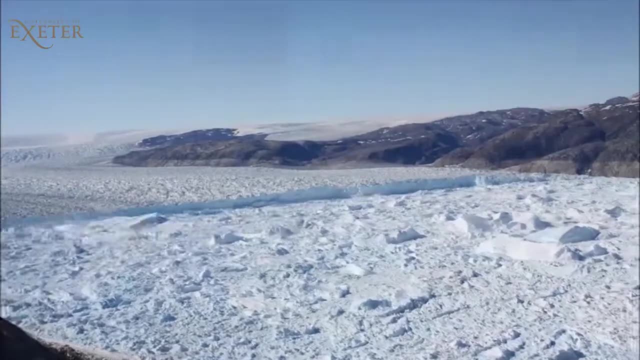 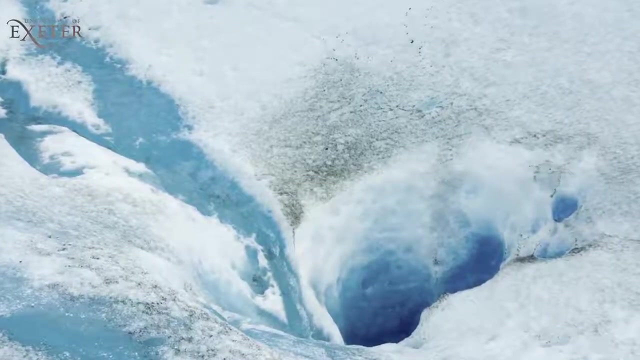 the reality is that Greenland has shown a very rapid response to warming over the past two decades. Ice loss has increased over this time, with glaciers showing an increase in flow speed and thinning of the ice. For Greenland, half of the total mass loss is from surface melt, whilst 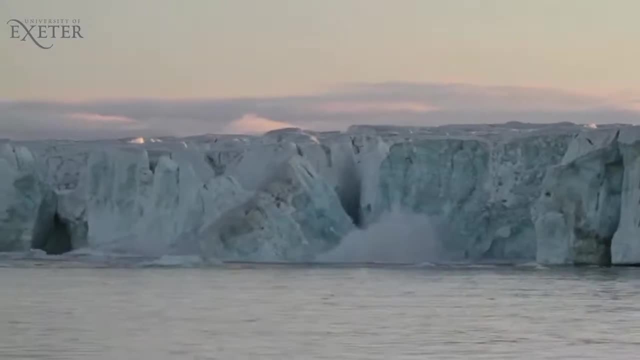 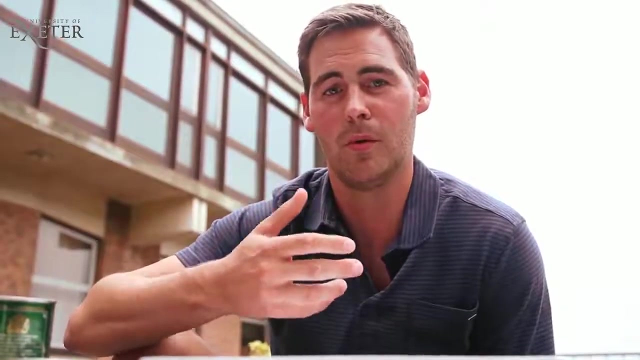 the remainder is due to blocks of ice breaking off, forming icebergs where the glacier meets the sea. This process is known as carving. So how do ice sheets move? Well, like all things, they tend to spread out under their own weight. Soft things like treacle will spread out easily. 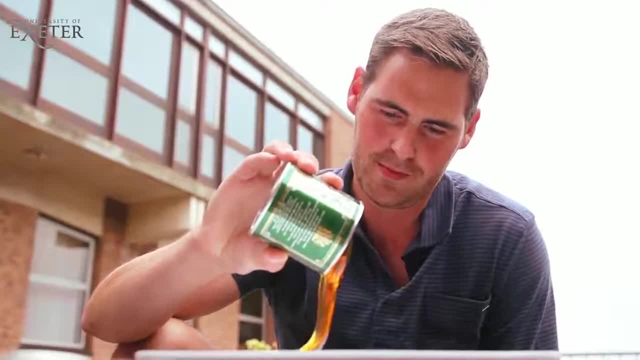 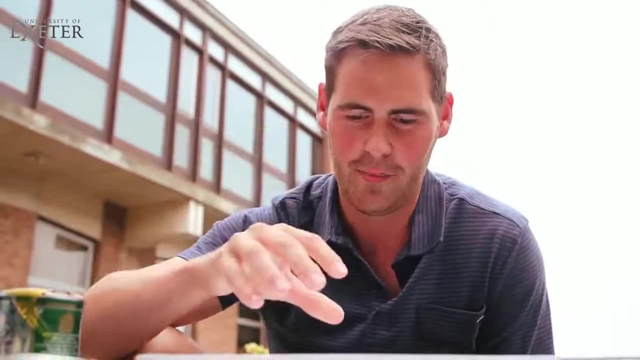 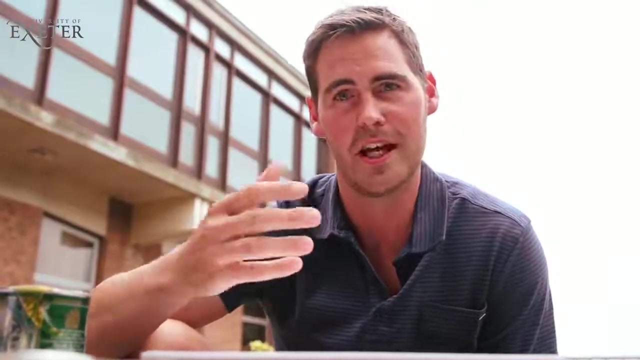 whereas strong things will resist spreading Ice sheets. ice sheets are piles of compressed snow that forms glacier ice. If it snows more, the pile will get larger and you have a positive mass balance If you increase the melt rate and it's larger than the amount of snowfall. 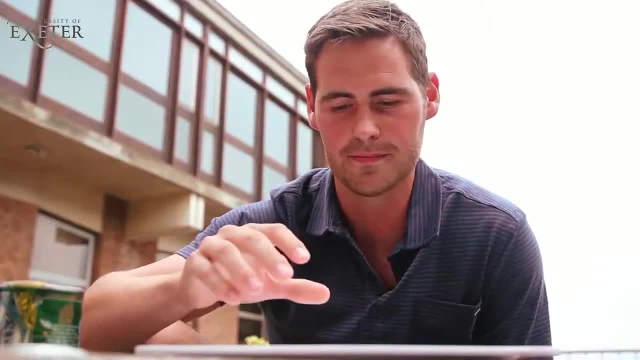 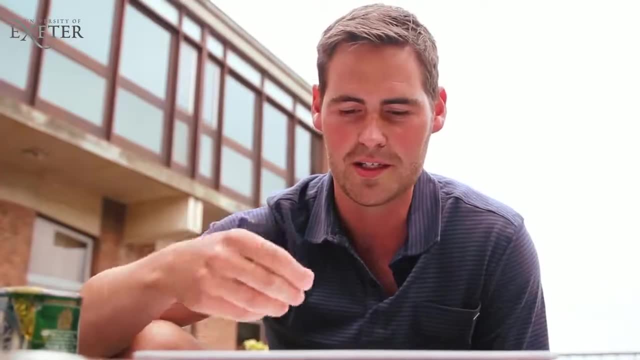 then you'll have a negative mass balance and the pile will get smaller. If the pile spreads faster, then more ice will get to the edges, and so the melting will increase. when you have more ice, So in the summer you'll have a larger amount of ice lost as iceberg carving. 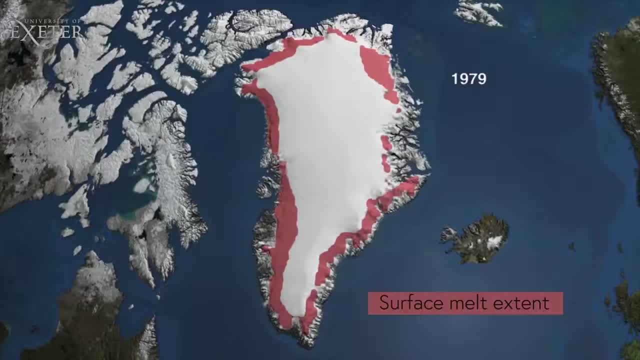 So let's look at these mass loss mechanisms in turn. On average, in the summer, about half of the surface of Greenland's ice sheet naturally melts At high elevations. most of that melt water quickly refreezes in place Near the coast. some of the melt water is retained by the ice sheet and the rest is lost to the ocean. 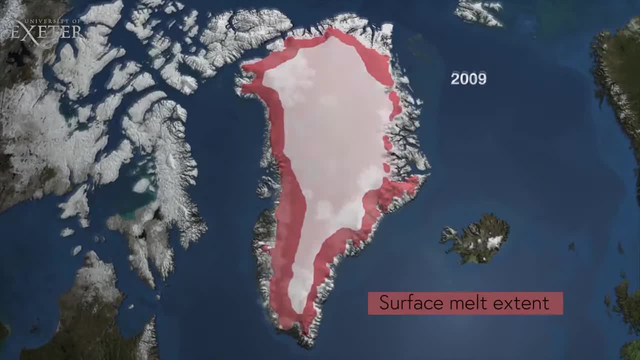 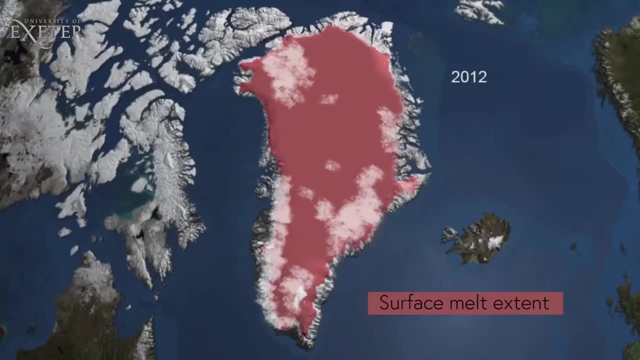 In 2012, nearly the entire summer experienced above normal melt extent across the coast, Across the Greenland ice sheet. much of this can be attributed to a shift in the regional scale patterns of high and low air pressure systems in the North Atlantic. Nonetheless, the melt extent 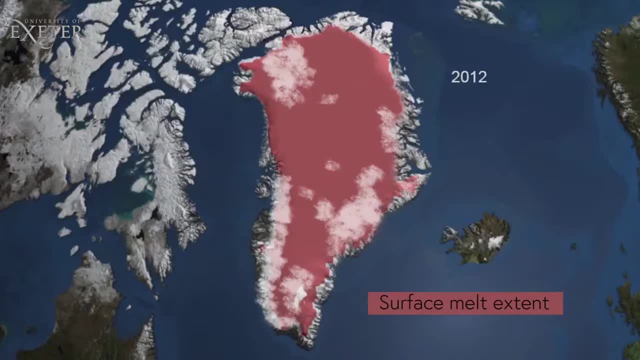 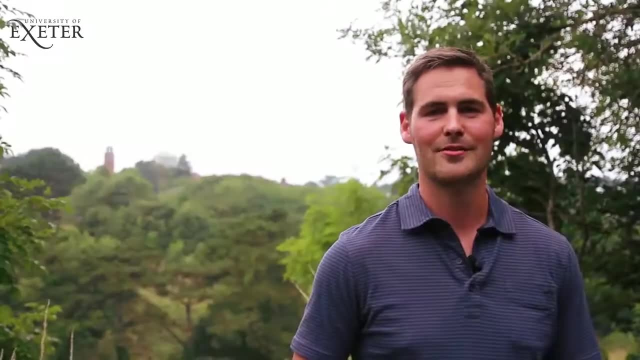 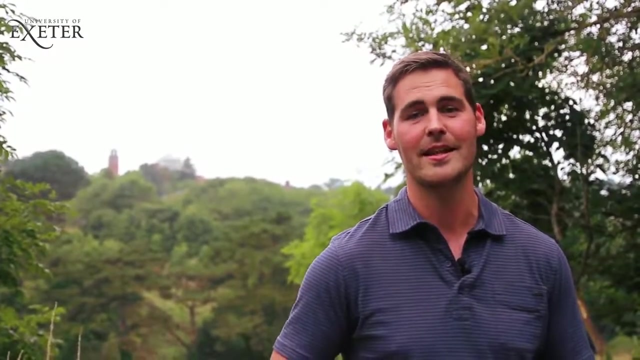 was the largest in the satellite era, extending up to 97 percent of the ice sheet surface and lasting two months longer than the 1979 to 2011 mean. Greenland may be near a tipping point. If the average annual temperature on Greenland increases by around three degrees celsius, then the ice sheet will rise. 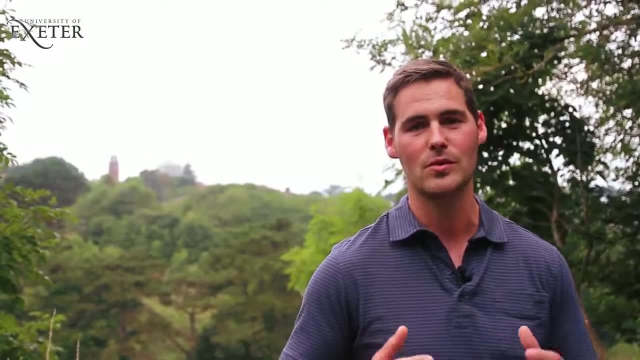 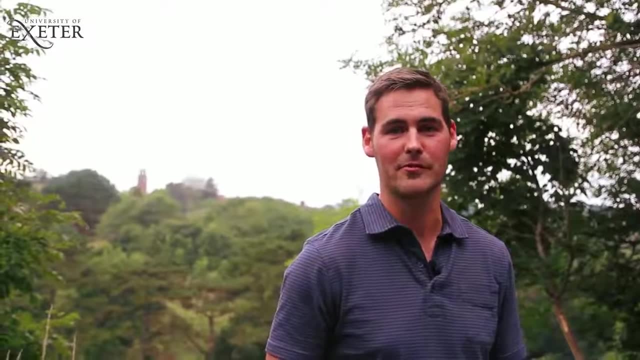 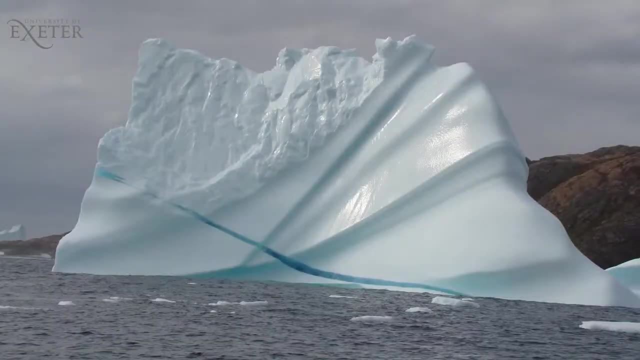 Then the ice sheet might melt at a rate which will tip it into a new, smaller inland form. But melt is only part of the story. Much of the increased mass loss from Greenland has resulted in an increase in ice flow or spreading, So more ice is flowing to the margins and is being lost. 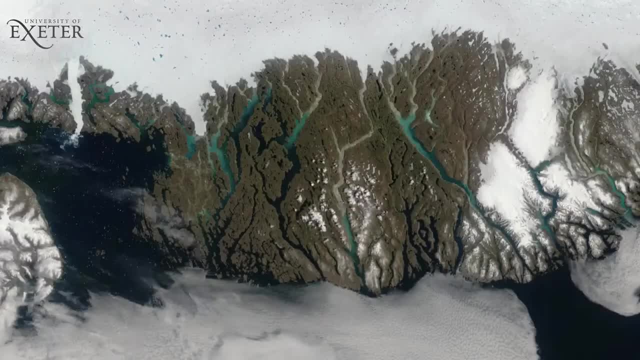 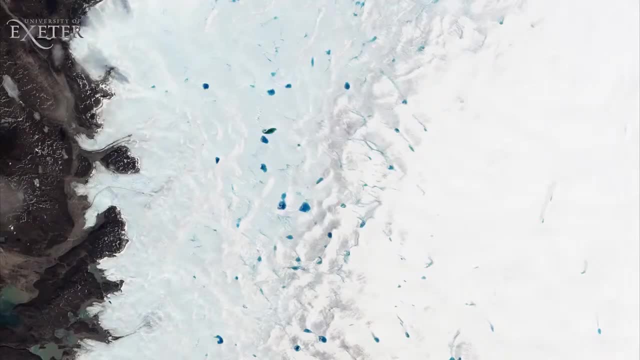 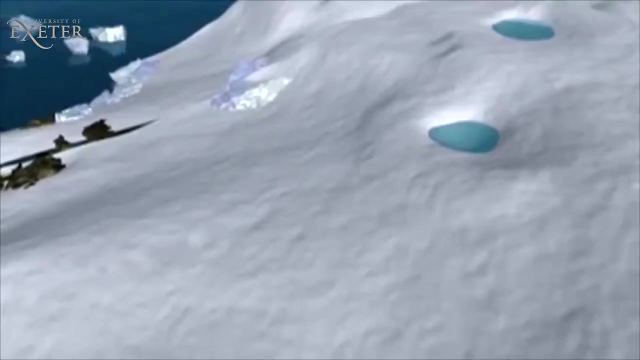 as icebergs. Basal lubrication occurs in Greenland when melt water drains to the bed Surface. melt water that hasn't drained to the bed or margins can collect in topographic depressions to form lakes. These lakes can be up to nine square kilometres in area and form all around. 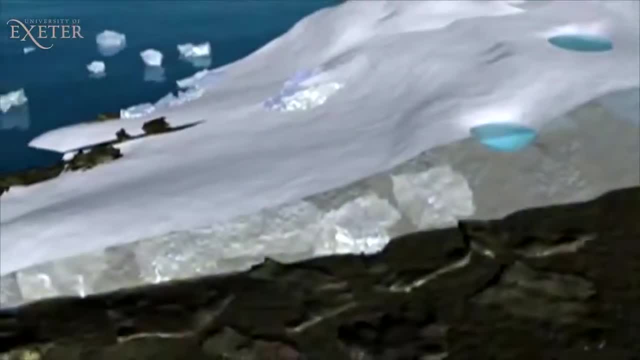 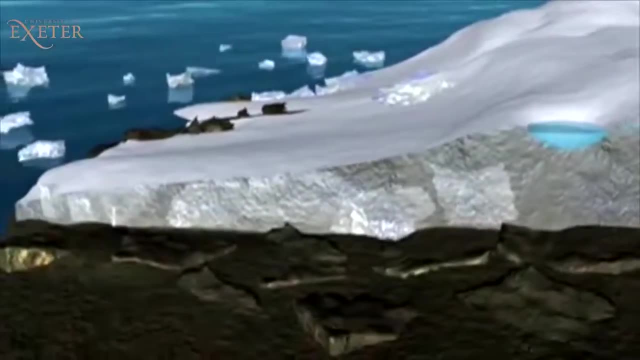 the edges of Greenland. Since the lakes are darker than the surrounding ice, they absorb more sunlight and so have a warming effect on the underlying ice. These lakes can drain abruptly, sending a substantial amount of melt water through the ice sheet to the bed. When the melt water reaches the 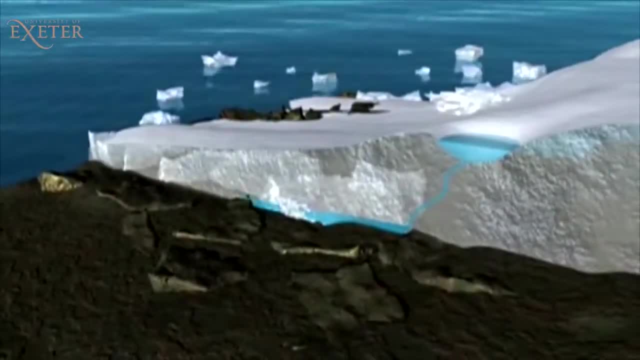 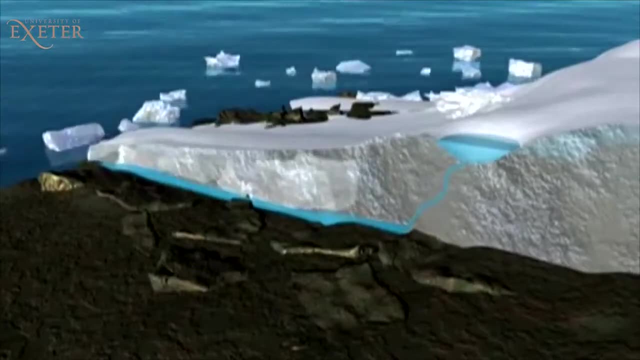 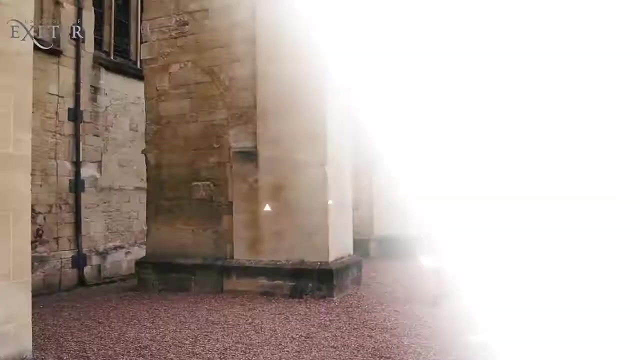 bed. it can have a lubricating effect on the ice sheet flow, causing short-lived acceleration events. In addition, the melt water transports heat to the interior of the ice sheet, which is warmer than the surrounding ice. This may have a warming effect on the ice sheet, softening it, allowing it to deform and flow faster. Another controlling process on ice: 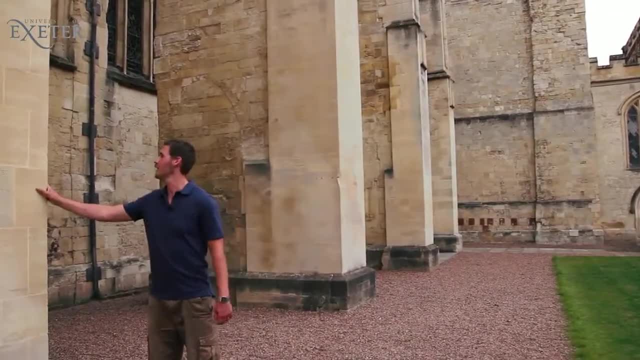 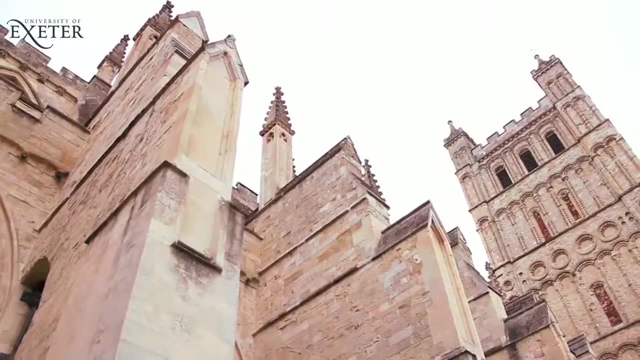 flow is buttressing which can oppose spreading. Just like the buttress on a cathedral holds the walls up, buttress around an ice sheet can resist ice flow. An ice sheet spreads under its own weight to the coast, where it either runs aground on a high spot in the bed, is topographically constrained. 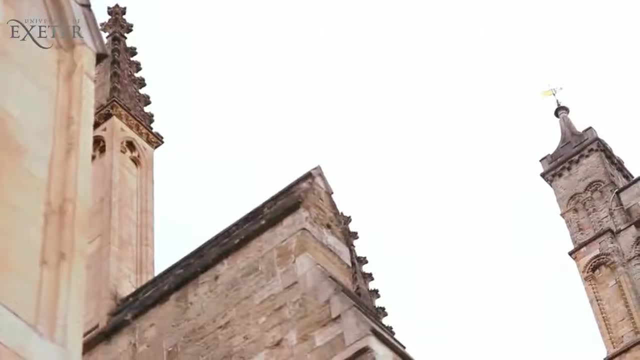 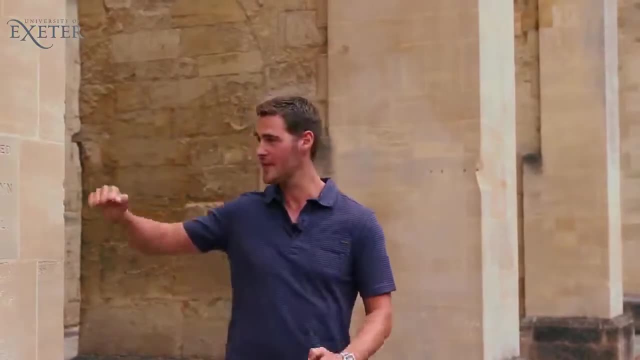 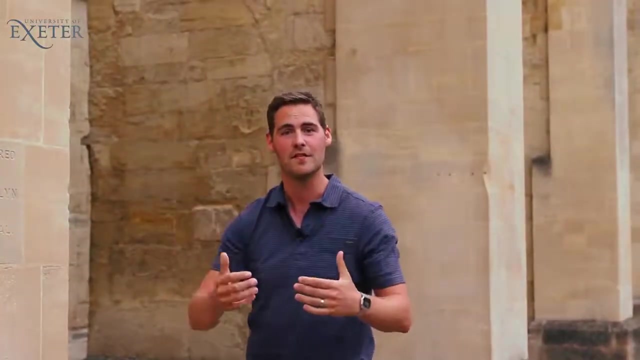 or flows over the ocean, creating a floating ice shelf. If you lose the floating ice shelf or retreat off a high spot in the bed, you remove this friction component which is effectively your flying buttress. The resistive stress is removed, which causes the feeding glaciers to flow faster and mass loss increases. 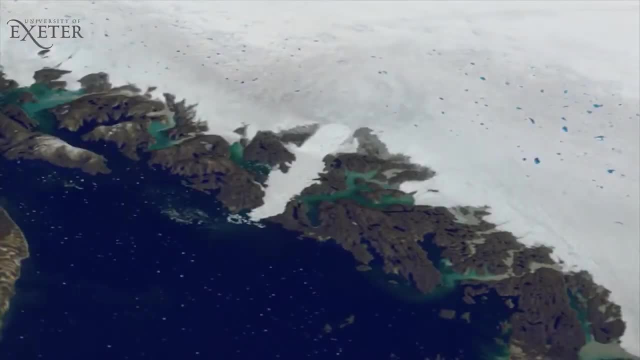 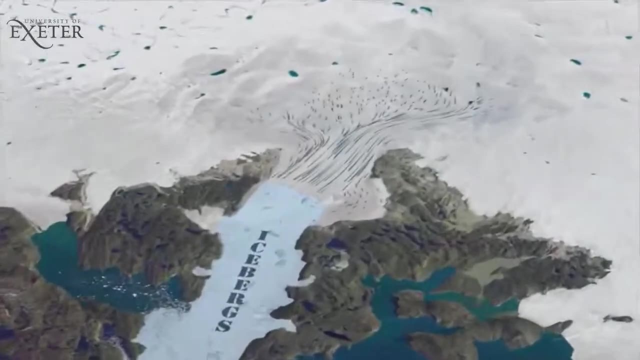 This is what happened on the west coast of Greenland at Jakobshavn, Isbray, one of the fastest flowing glaciers in the world. On the left of the animation is floating ice made out of icebergs and sea ice. On the right is the ice cliff where the terminus of the glacier meets.